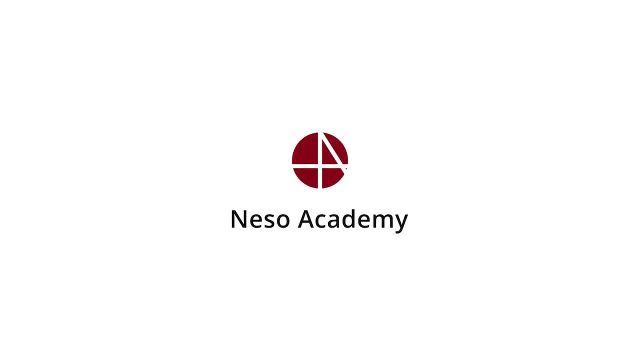 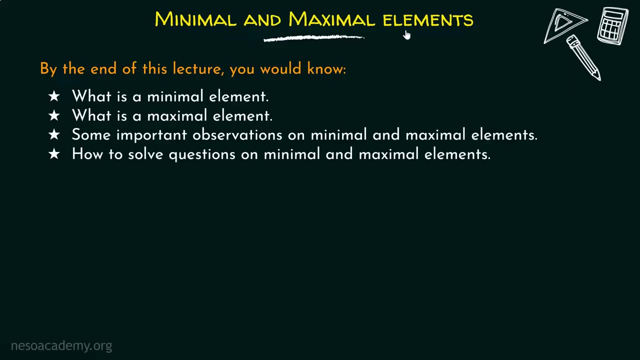 In this presentation we will discuss what is a minimal and maximal element. By the end of this lecture, you would know what is a minimal element, what is a maximal element. some important observations on minimal and maximal elements. how to solve questions on minimal and maximal elements. 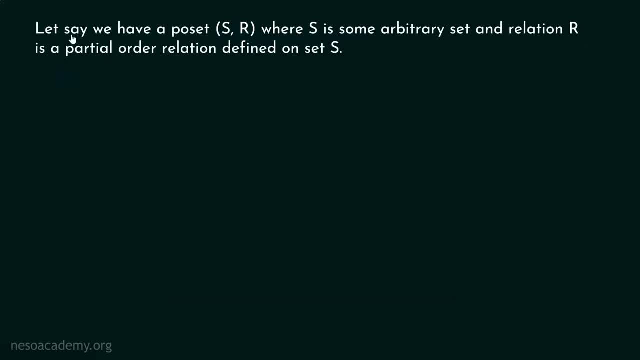 So, without any further delay, let's get started. Let's say we have a poset S R where S is some arbitrary set and relation R is a partial order relation defined on set S. So we have a poset S R and S is some arbitrary set. 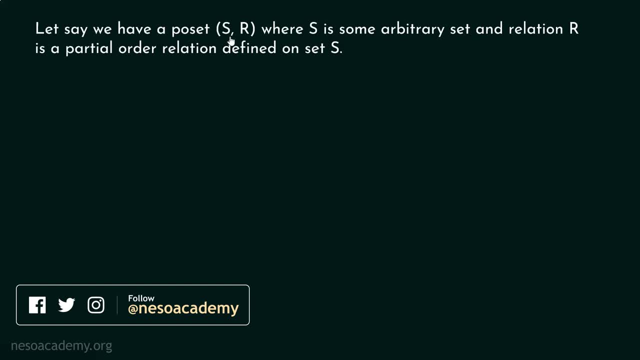 R is relation defined on this set and R must be a partial order relation. Okay, This is the definition of minimal element. An element x of a set, S, is called a minimal element. if there is no y belongs to S, such that y is related to x, or in other words: 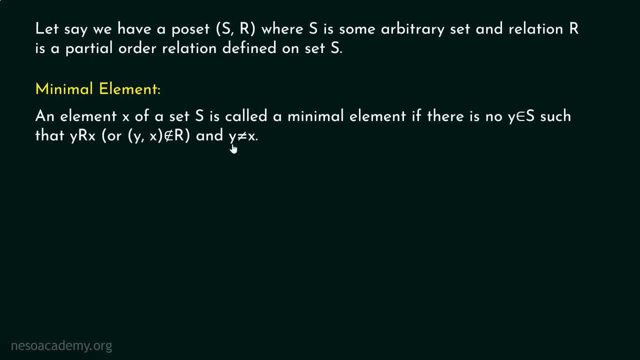 y comma. x does not belong to R, And it must be well noted that y must not be equal to x. This is quite a simple definition to understand, if we see this carefully. Here we are talking about some element x, Okay, And this element must belong to set S. 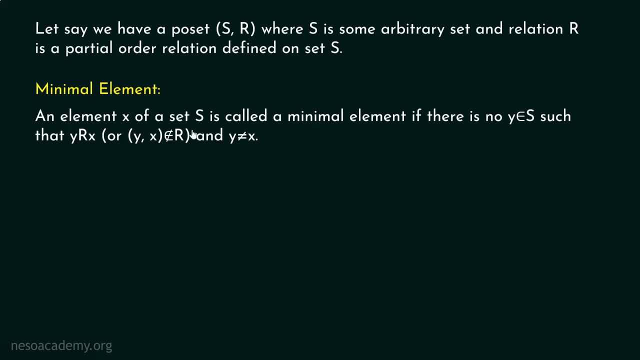 Apart from this, we are saying that this element is called a minimal element. if there is no y belongs to S, such that y is related to x, Okay, There must not be any y belonging to S, Such that y is related to x. 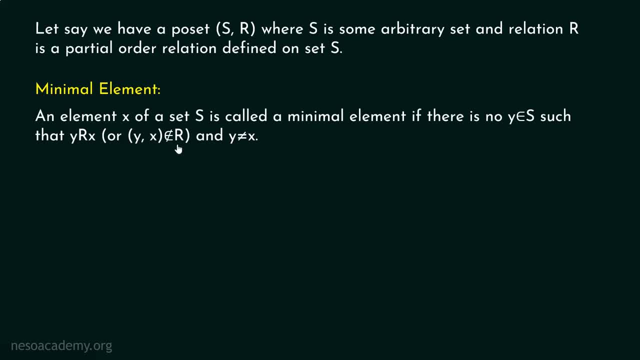 Or in other words, we can say y comma. x must not belong to R, And it must be well noted that y must not be equal to x. Okay, We know that x is related to itself. That's why I am saying that y and x must be different. 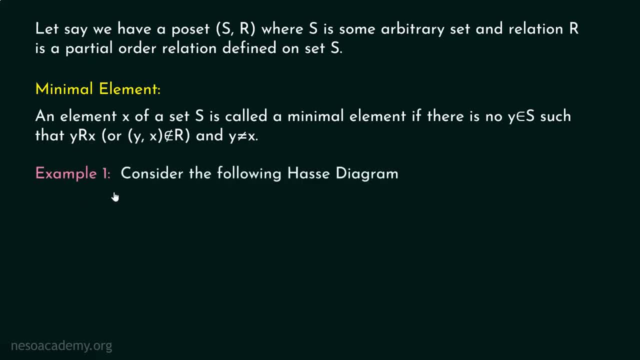 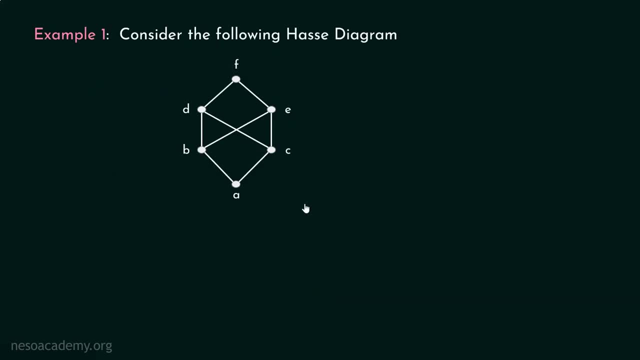 They must not be identical. Okay, Now here is one example. Let's consider the following Hess diagram. This is our Hess diagram. And now what I want to do? I just want to find all the minimal elements in this Hess diagram. This Hess diagram is obviously representing some partial order. 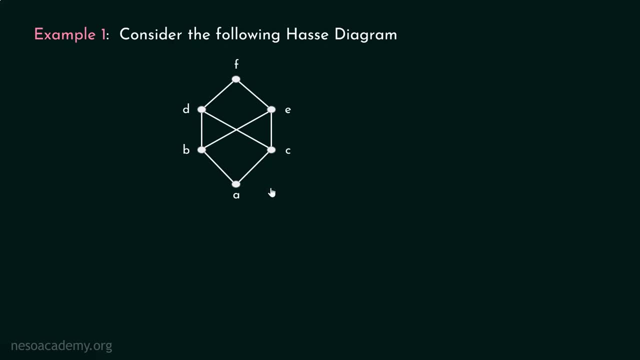 Right Here. I am interested in finding all the minimal elements. Fine, So let's just find them out. In the above Hess diagram, b and c are not minimal, because a is related to b and a is related to c. If you see this, then b and c are not minimal elements. 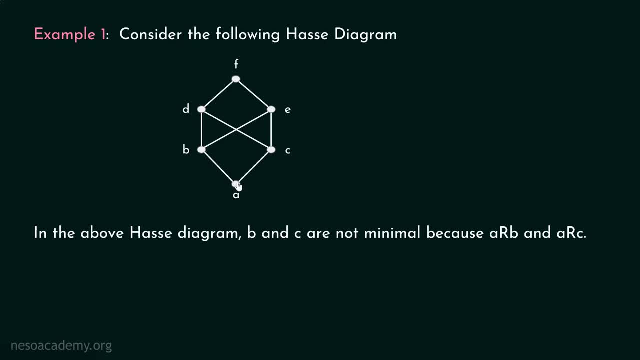 because a is related to b and a is also related to c. According to the definition, x is a minimal element if there is no y, such that y is related to x. Here you can see that a is related to b. How can we say that b is a minimal element? 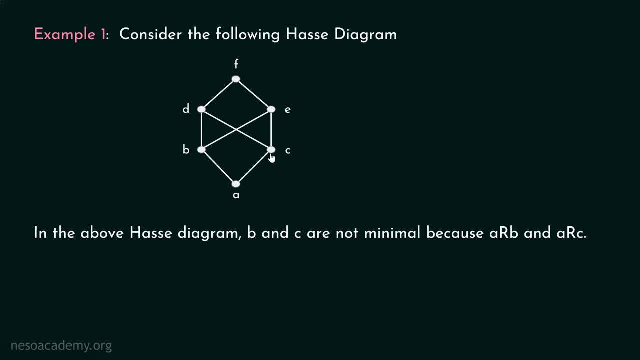 Right. Similarly, we cannot say that c is a minimal element because a is related to c. Apart from this, d and e are not minimal because b is related to d and c is related to d. Also, c is related to e and b is related to e. 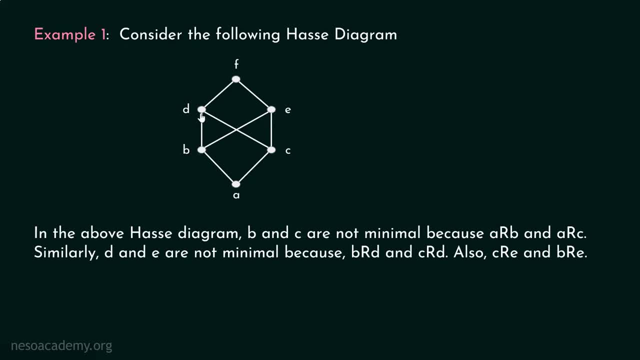 You can see that d and e are also not minimal because b is related to d, c is related to d, D, E is also not a minimal element because B is related to E and C is related to E, right. Also, F is not a minimal element because D is related to F and E is also related to F. 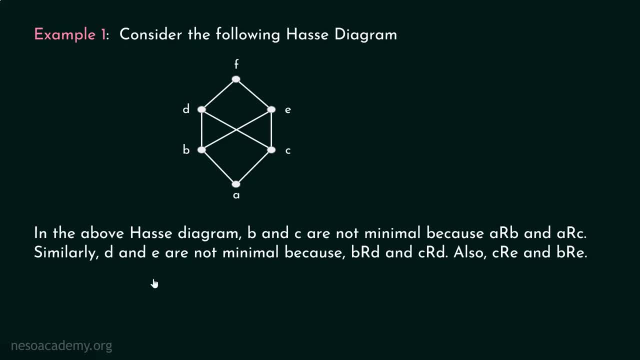 But if you see this Hess diagram, A is the minimal element, right? A is the only minimal element, because no element is related to A. There is no element below this element which is related to this element, right? No element is related to A. Therefore, A is the only. 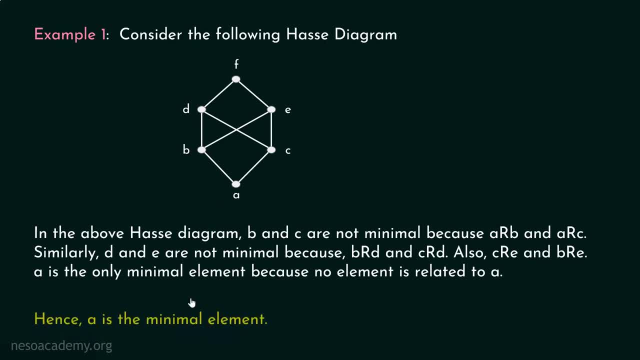 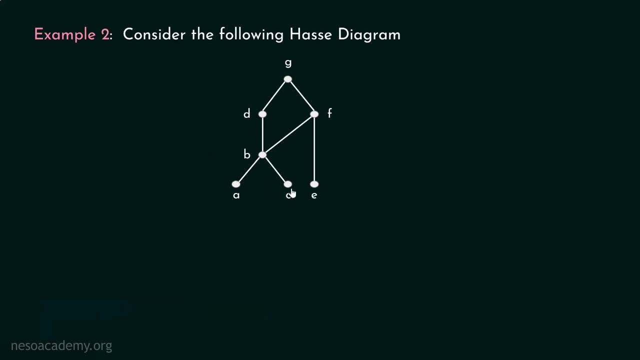 minimal element in this Hess diagram, right. Hence, it is clear that A is the only minimal element. right Now let's consider example 2.. In this example, let's consider this Hess diagram. Here, in this Hess diagram, we have all these vertices and the edges drawn between 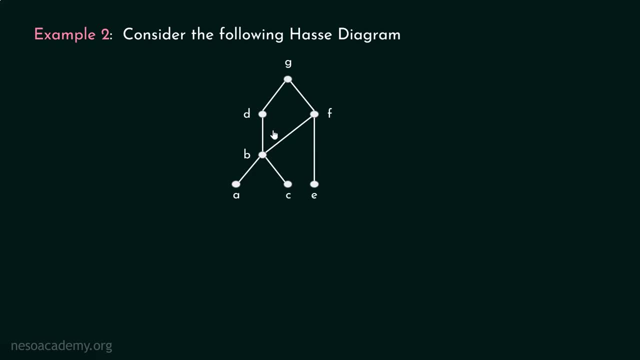 them right Now. we have to identify the vertices. Now we have to identify what are the minimal elements in this Hess diagram. In the above Hess diagram, A, C and E are minimal because no element is related to A, C and E. If you see this carefully, then A, C and E are minimal elements because there 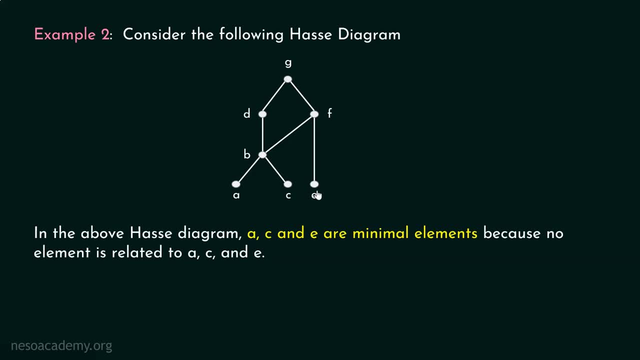 is no such element which is related to these elements, right? So it is clear that A, C and E are minimal elements, right? It is quite easy to identify the minimal elements from the Hess diagram. That is why Hess diagrams are quite clear. 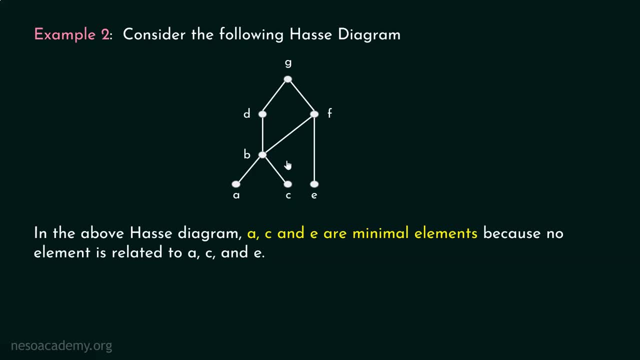 It is quite useful, right? So finding the minimal elements is quite easy from the Hess diagrams, and that's why I have chosen Hess diagrams to find the minimal elements of a particular partial order. okay, Now there is one important observation: A poset can have more than one minimal element. 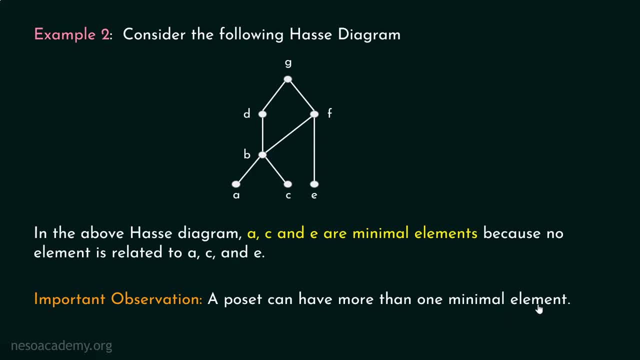 okay, This is very true. A poset can have more than one minimal element. You can see this: that in this Hess diagram there are total three minimal elements. Obviously, it is clear that a poset can have more than one minimal element. Now we will discuss. 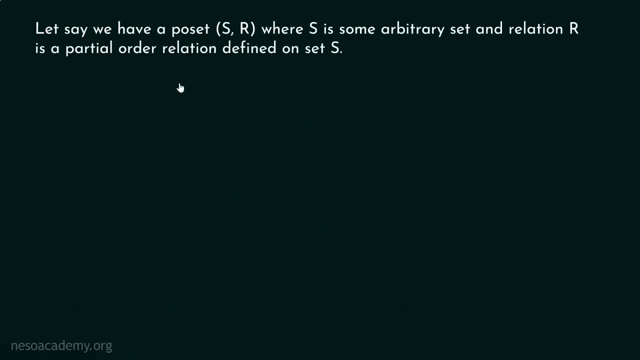 the definition of maximal elements. Again, I am considering the poset, where S is some arbitrary set and R is a relation defined on this set, which is nothing but a partial order relation right. An element x of a set, S, is called a maximal. 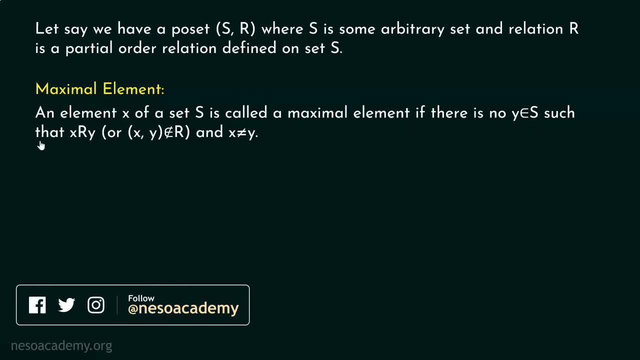 element. if there is no y belongs to s, such that x is related to y, Or in other words x comma. y must not belong to R And obviously x must not be equal to y. This is very true, right. The definition is little bit changed. 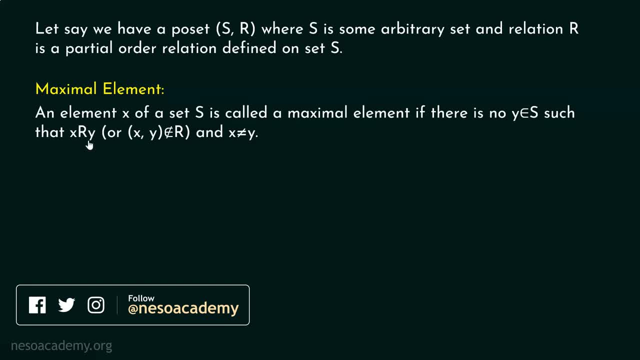 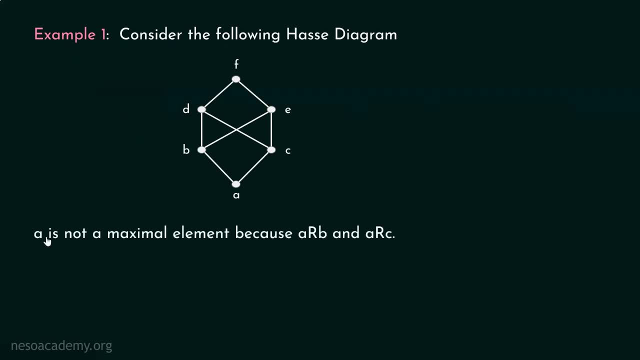 Here, instead of y related to x, we have x related to y. We will understand this with the help of an example. Let's consider the following Hess diagram. In the above Hess diagram, a is not a maximal element, because a is related to b and a is related to c. 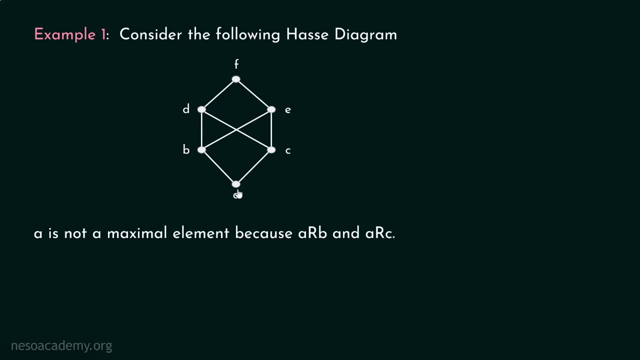 If you see this, this element is not a maximal element, Because this element is related to b and this element is related to c. According to the definition of maximal element, x is a maximal element if there is no y belongs to some set S. 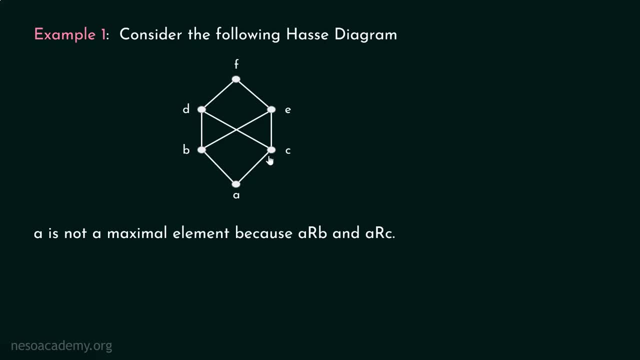 on which the relation is defined, x must not be related to y. Right, Then only we can say that x is a maximal element. Right, We must consider every y of set S other than element x. Right Here you can see that a is not a maximal element. 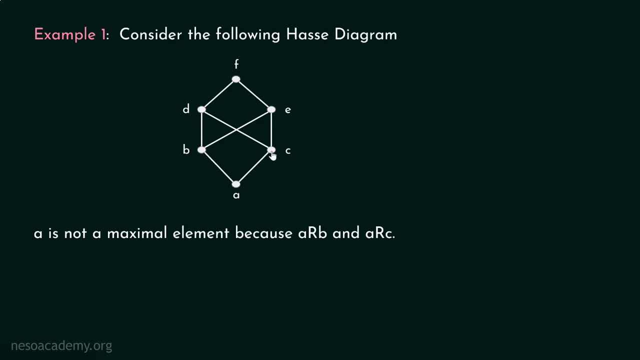 because a is related to b and a is related to c. Apart from this, b, c and e are not maximal elements, because b is related to d and b is related to e. c is related to d and c is related to e. 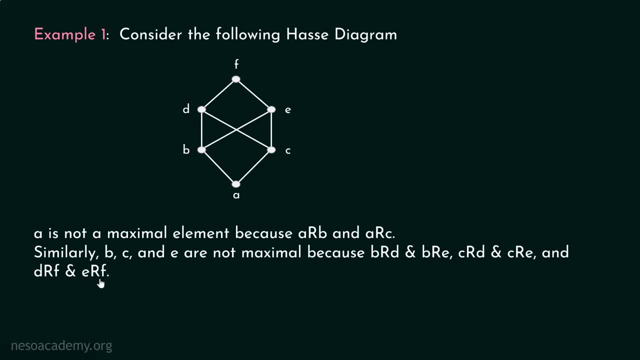 Also, d is related to f and e is related to f. Right b is related to d, b is related to e, c is related to d, c is related to e, d is related to f and e is related to f. 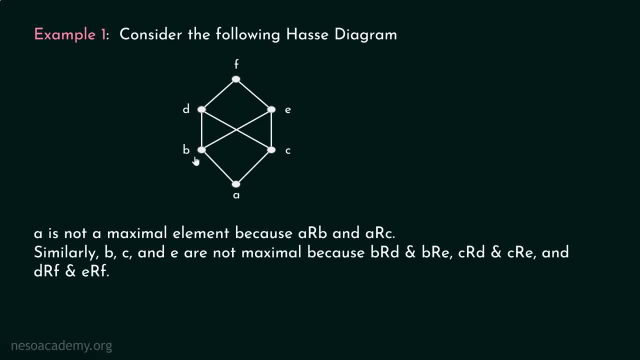 Right. It is clear that all these elements are not maximal, except element f. Right, f is the only maximal element, because f is not related to any element. Therefore, it is clear that f is the maximal element. Hence it is clear that. 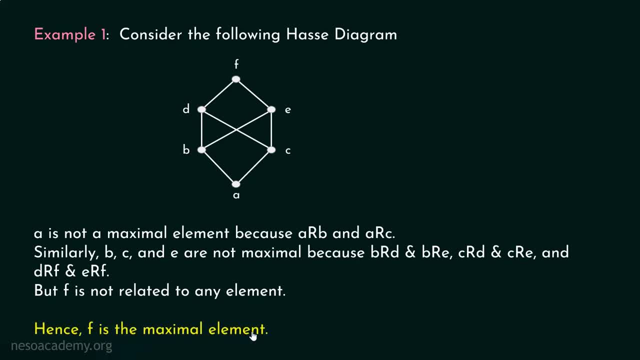 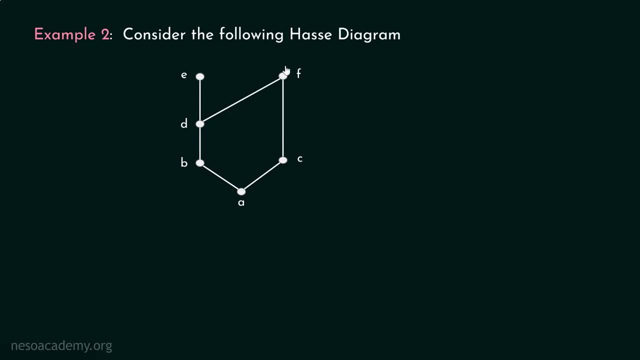 f is the maximal element. There is no doubt about this. Right Now, let's consider example 2.. Consider this Hess diagram. Now we want to find what are the maximal elements in this Hess diagram, In the above Hess diagram. 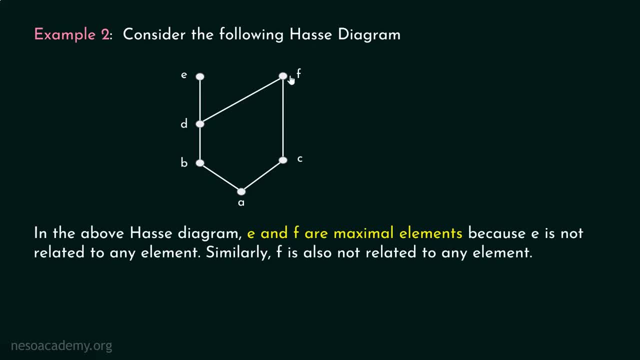 e and f are maximal elements. You can see that e and f are maximal elements. Again, it is easy to identify all the maximal elements in a Hess diagram. e and f are clearly the maximal elements because e is not related to any element. 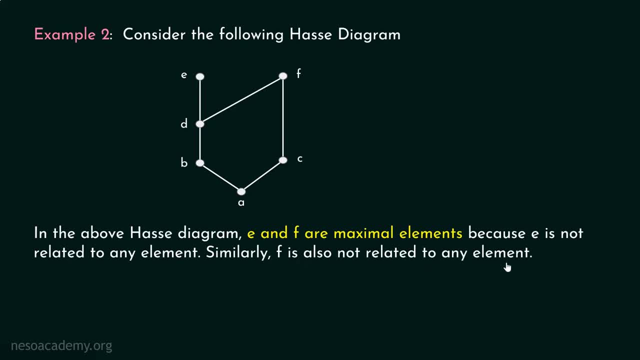 Similarly, f is also not related to any element. Right Again, there is one more important observation. A poset can have more than one maximal element. There is no doubt about this. From this Hess diagram, it is clear that a poset can have more than one maximal element. 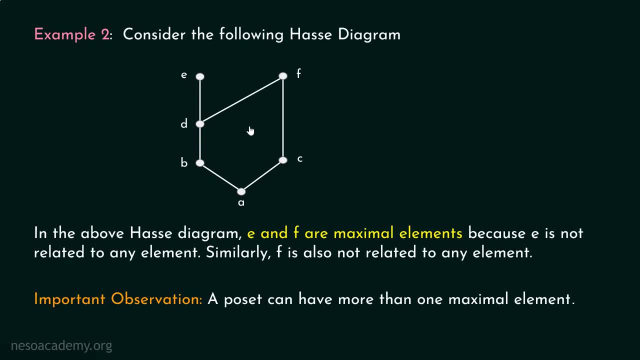 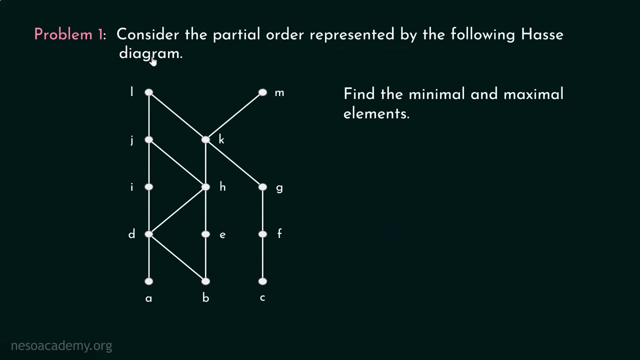 Right, So there can be more than one minimal as well as maximal element. There is no doubt about this. Right Now, we will consider some problems related to maximal and minimal elements. Here is problem 1.. Consider the partial order represented by the following Hess diagram: 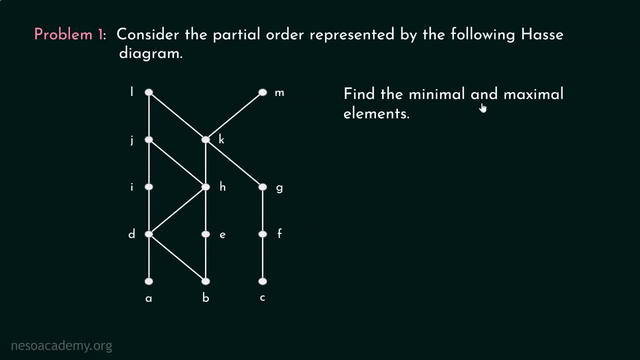 This is the Hess diagram available with us. We have to find the minimal and maximal elements from this Hess diagram. Okay, Here is the solution. Maximal elements are l and m. You can see these are the maximal elements, Right, Because l is not related to any other element. 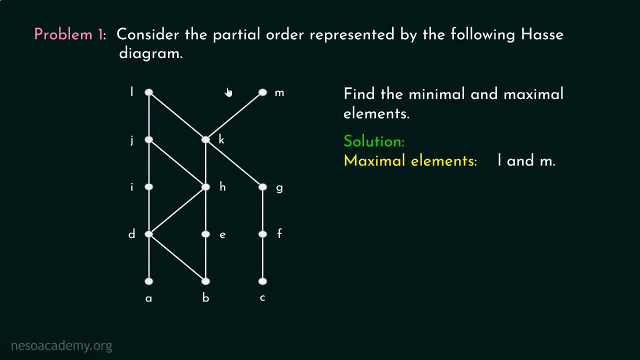 and m is also not related to any other element. There are no elements above these elements. Therefore, these are the maximal elements. Right Apart from this, the minimal elements are a, b and c. If you see this diagram carefully, a, b and c are the minimal elements. 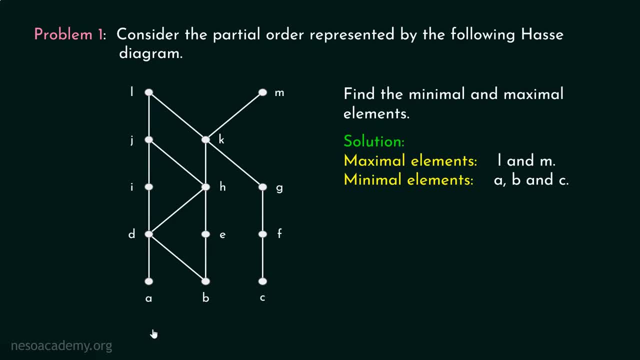 Because there are no elements below these elements which are related to these elements. Right, Therefore, these are minimal elements. So maximal elements are l and m and minimal elements are a, b and c. Fine, Now let's consider problem 2.. 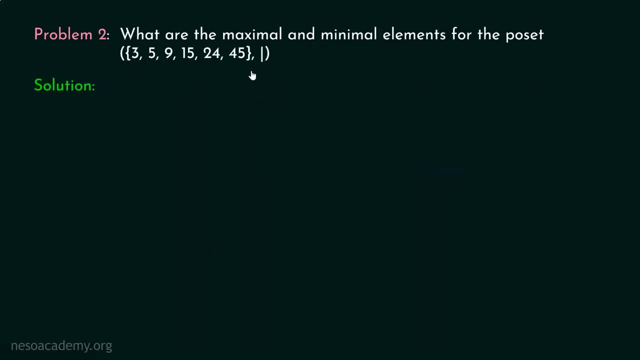 What are the maximal and minimal elements for this poset? We have to identify maximal and minimal elements for this particular poset. The best option is to draw the Hess diagram for this poset. Okay, Here you can see: relation is divides relation. 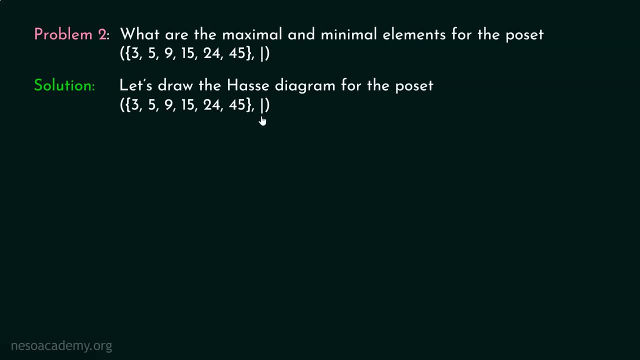 Right. So we have some imaginary relation r, which consists of ordered pairs- a- b, such that a divides b Right, And the relation must be defined on this particular set. You can see that 3 and 5 are incomparable and no element divides 3 and 5.. 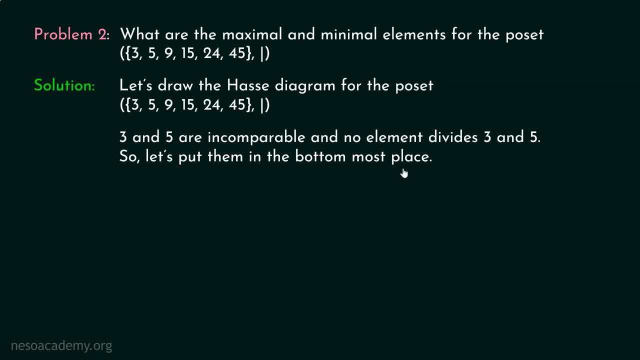 Right, So let's put them in the bottom most place. 3 and 5 are incomparable, So let's just put them in the bottom most place, because they are incomparable and no element divides 3 and 5.. Apart from this, 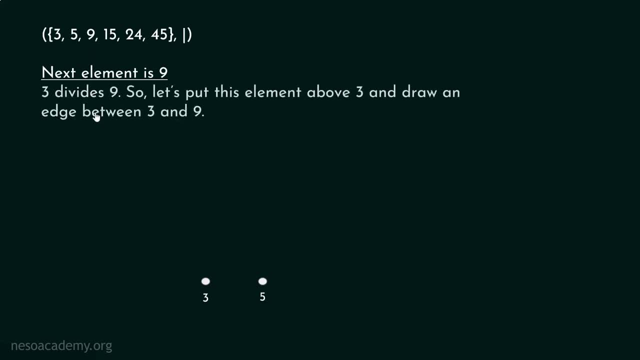 the next element is 9. in this set Right, 3 divides 9.. So let's put this element above 3 and draw an edge between 3 and 9.. Why can't we just put this element 9 above 3?? 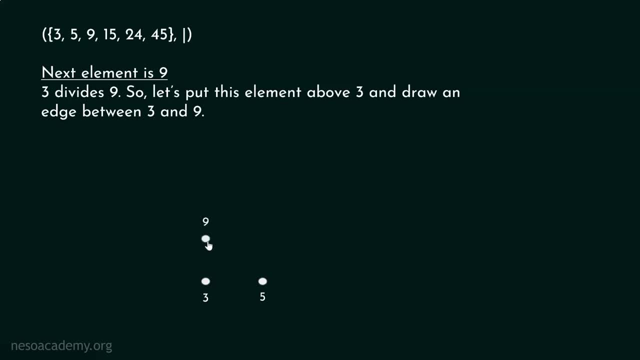 Because 3 divides 9.. So let's just put this element above 3 and let me just draw an edge between 3 and 9, because 3 divides 9.. Right, And you must note this, that 5 does not divides 9.. 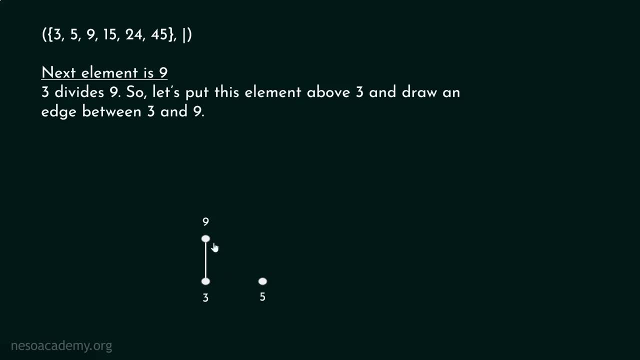 Therefore, we cannot place an edge between 5 and 9.. Right After this, the next element is 15 in this particular set. Now let's just place it somewhere, But before placing it, we can see that the top elements are 9 and 5.. 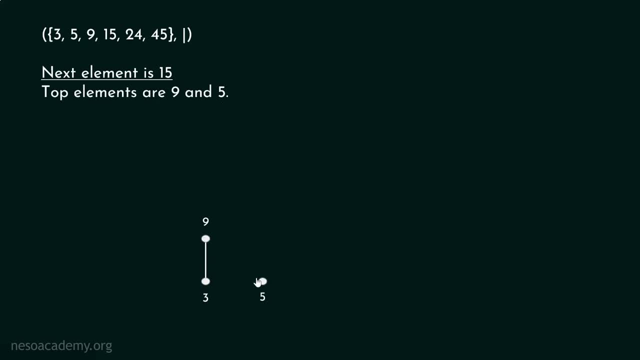 Right Here in this figure, 9 and 5 are the top elements. So we must see whether 15 is divided by 9 or 5.. Okay, 9 does not divide 15.. But 3 and 5 divides 15.. 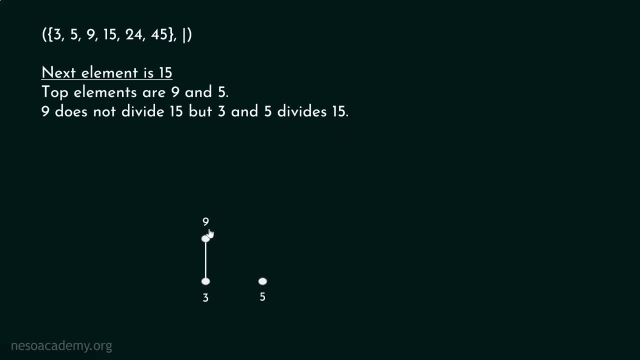 Right, This element 9 does not divide 15.. After checking whether 9 divides 15 or not, we have seen that 9 does not divides 15.. Therefore, we will move one step below And here you can see we have element 3.. 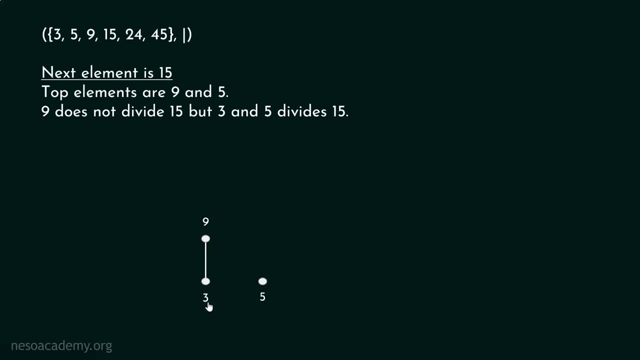 So we will check whether 3 divides 15 or not, And we know that 3 divides 15.. Apart from this, 5 also divides 15.. So let's draw an edge between 3 and 15 and 5 and 15.. 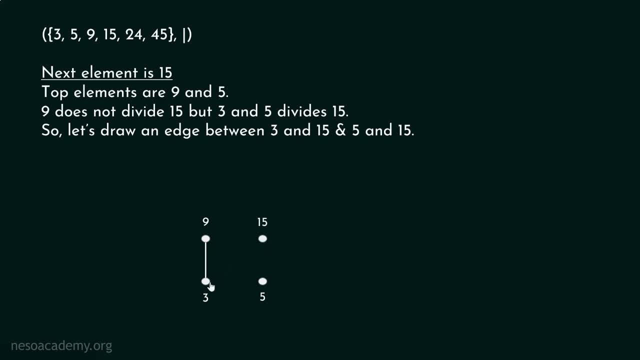 Right. So let me place 15 over here And let me draw an edge between 3 and 15 and 5 and 15.. Right After this, the next element is 24.. Top elements are 9 and 15.. 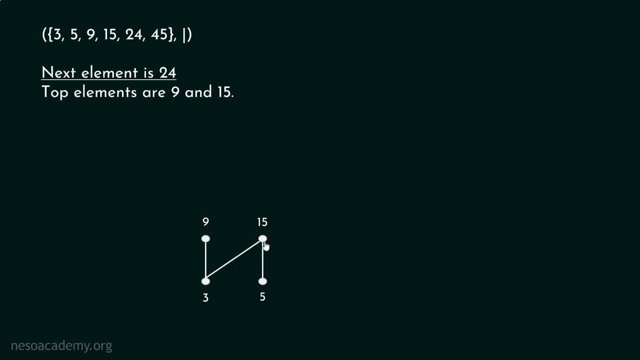 You can see that in this figure 9 and 15 are top elements Right. 9 does not divide 24.. We know that 15 does not divide 24.. But 3 divides 24.. 9 does not divide 24.. 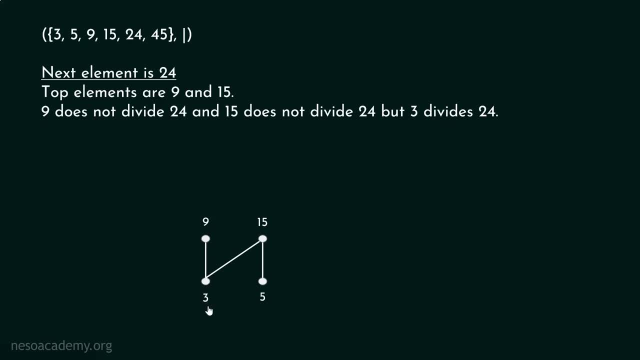 Therefore, we will go one step below And we can see that we have an element: 3.. 3 does divides 24.. Also, 15 does not divide 24.. And it is also true that 5 also does not divide 24.. 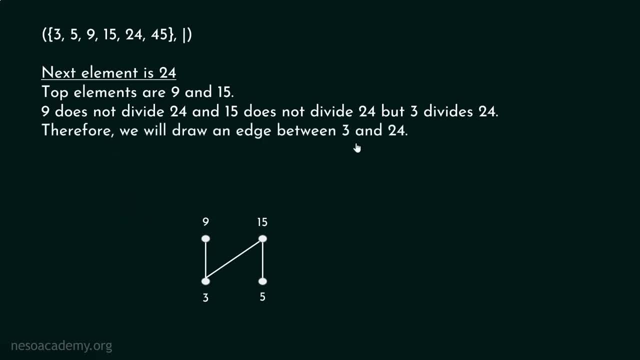 Therefore, we will place an edge between 3 and 24.. Right, So let me just draw the vertex over here And let me just place an edge between 3 and 24.. After this last element is 45.. Top elements are 24,, 9 and 15.. 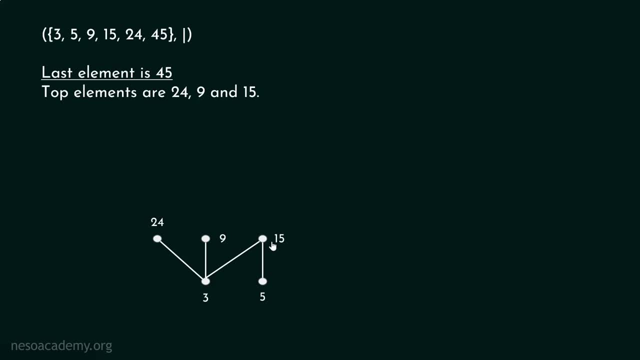 You can see 24, 9 and 15 are the top elements. 24 does not divide 45. But 9 divides 45.. 24 does not divide 45. But 9 divides 45. Also, 15 divides 45.. 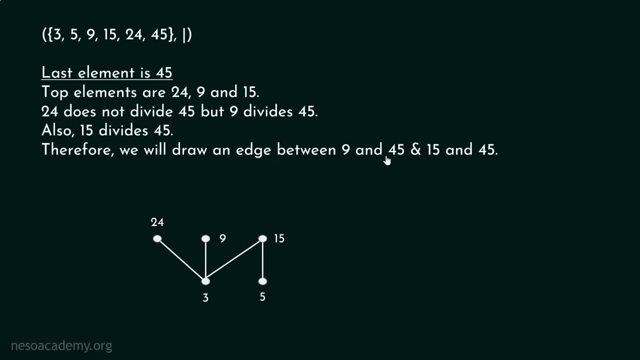 Therefore, we will draw an edge between 9 and 45 and 15 and 45.. So let me just place this vertex 45 over here And let me draw an edge between 9 and 45 and 15 and 45..